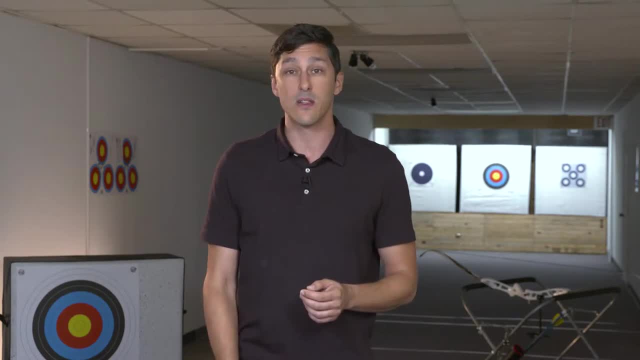 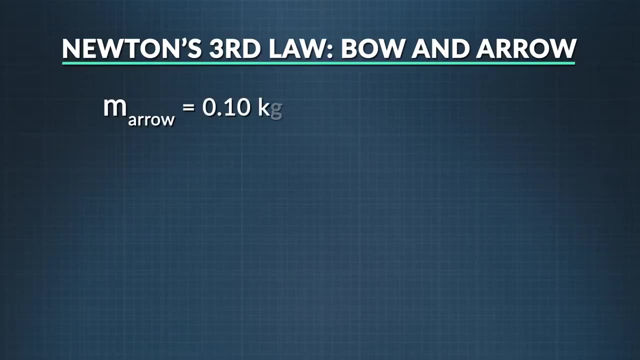 not the mass of the arrow. Let's figure out how much the bow will accelerate back as the arrow is launched forward into the air. The arrow has a mass of 0.10 kilograms, with an average rate of acceleration of 1,280 meters per second squared. 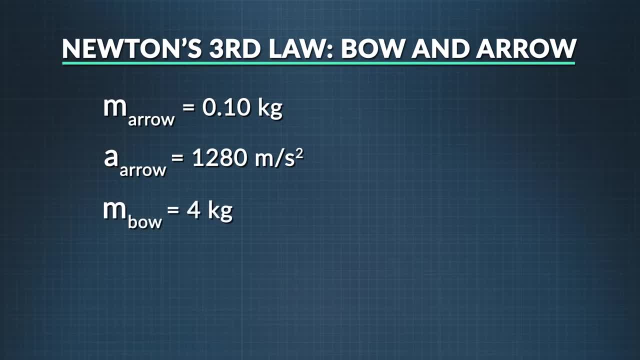 The mass of the bow is 4 kilograms. The bow exerts a force on the arrow as it is fired in the positive x direction. According to Newton's third law, the bow will also experience a force from the arrow of equal magnitude in the negative x direction. 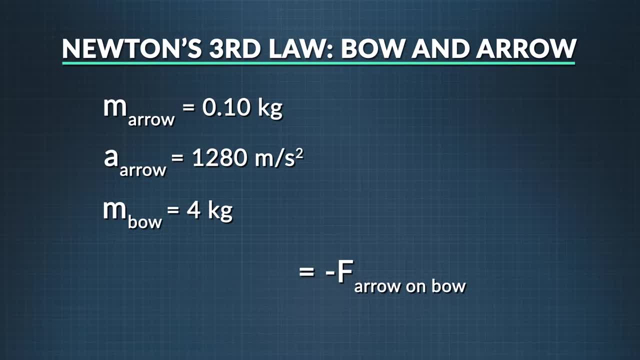 We see that by substituting in Newton's second law, the mass of the arrow times the acceleration of the arrow equals the mass of the bow times the acceleration of the bow in the opposite direction. We can rearrange this equation to solve for the acceleration of the bow. 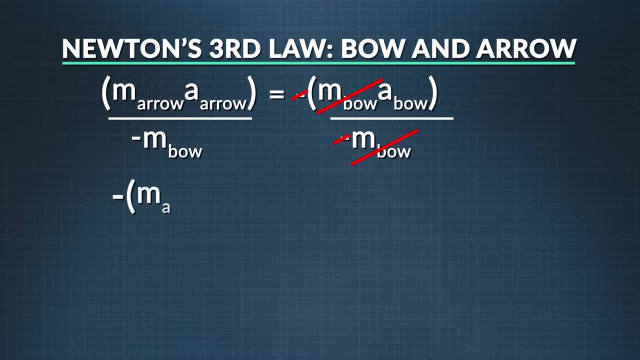 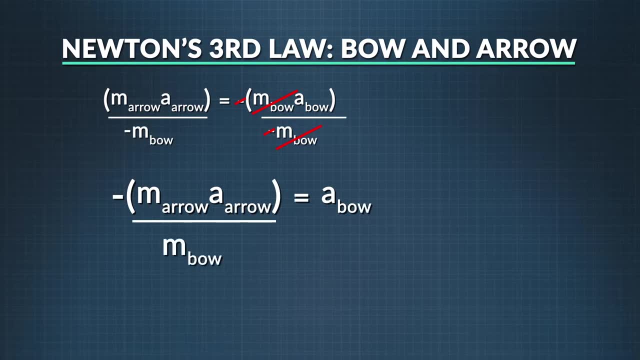 The acceleration of the bow equals negative. the mass of the arrow times the acceleration of the arrow divided by the mass of the bow. We can now plug in our values to find the acceleration Negative: 0.10 kilograms times 1,280 meters per second squared. 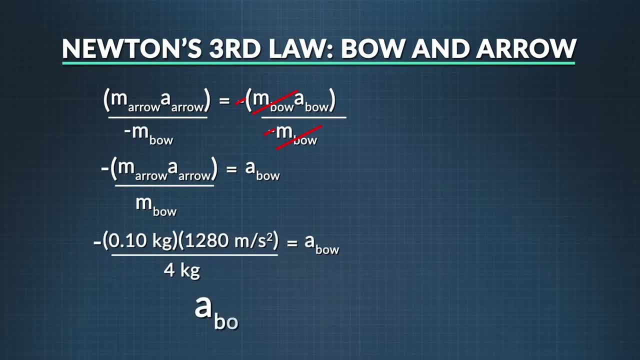 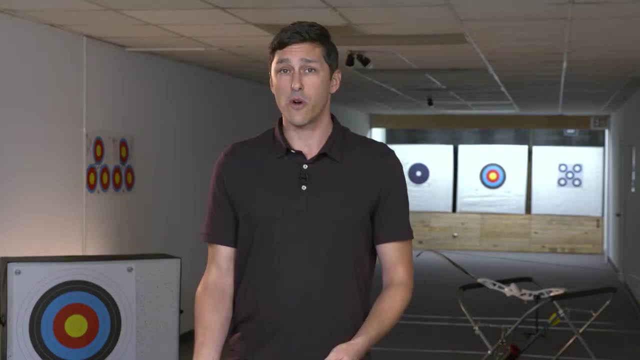 divided by 4 kilograms equals negative 32.0 meters per second squared, or 32.0 meters per second squared in the negative direction. Thus the bow accelerates backwards at 32.0 meters per second squared. If the force of one thing acting on another is always equal in magnitude. 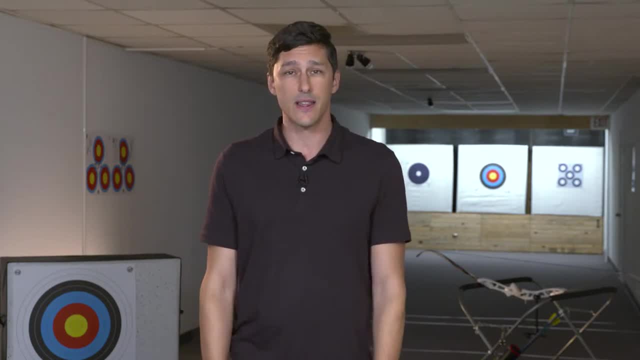 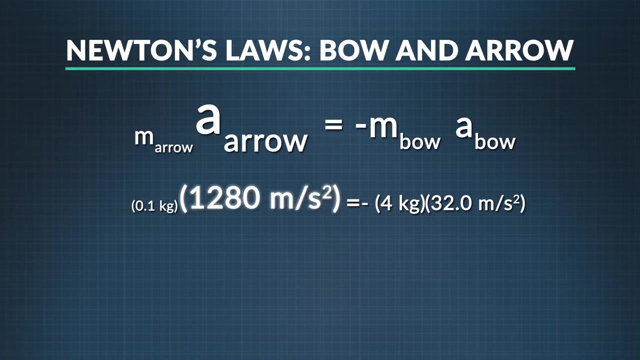 yet opposite in direction. then how does anything ever accelerate? Even though the two forces are equal in magnitude, one can accelerate more than the other because one can have a smaller mass, like the arrow. when compared to the bow, The much smaller arrow accelerated at 1,280 meters per second squared. 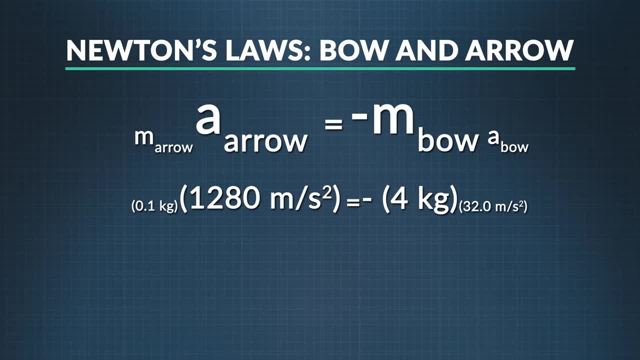 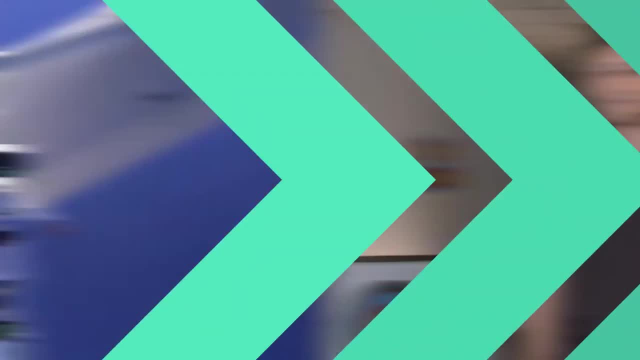 while the much larger bow accelerated at a smaller amount: 32.0 meters per second squared. Okay, let's head for the skies and look at another example. A skydiver is in a freefall toward Earth. The Earth is pulling the skydiver with the same force. 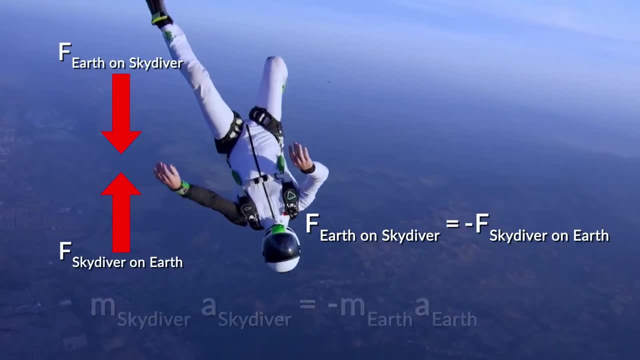 as the skydiver is pulling on the Earth, but in the opposite direction, Even though the forces are the same. the skydiver is accelerating to Earth exponentially faster than the Earth is accelerating toward the skydiver, Because Earth is so much more massive. 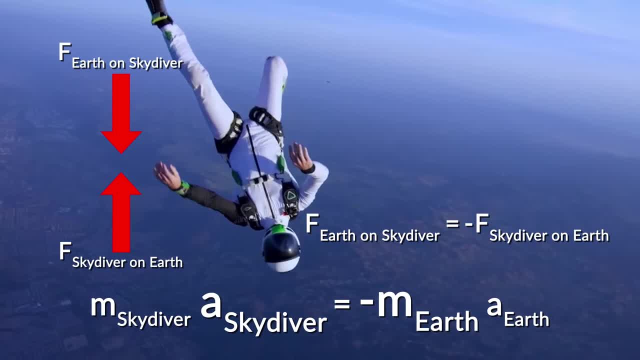 it takes a lot more force to move the Earth compared to the skydiver, So the acceleration isn't the same and neither is the mass. So each side of the equation is equal, but the variables on each are bigger or smaller depending on the mass and acceleration of the objects. 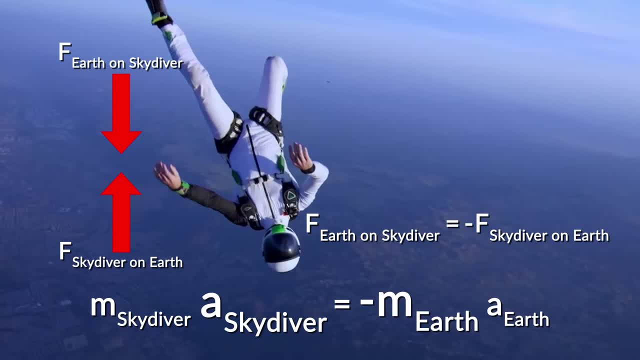 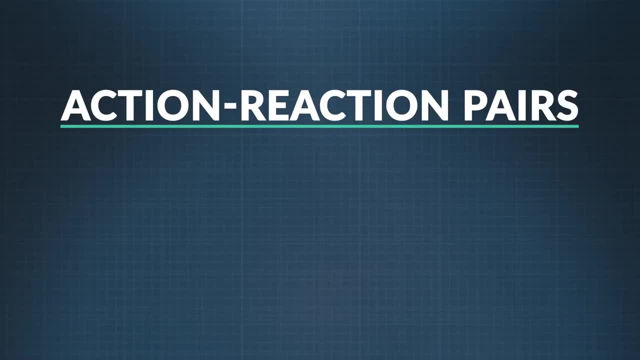 As far as physics goes, and following Newton's third law, the Earth does accelerate toward the skydiver ever so slightly. We can sum up this idea into what's called an action-reaction pair. Action-reaction pairs show the relationship between an object. 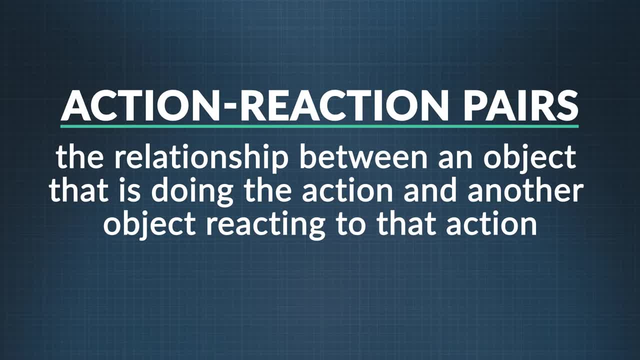 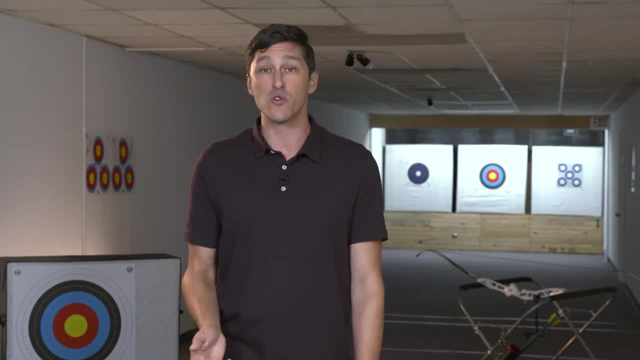 that is doing the action and another object reacting to that action. As a skydiver jumps from a plane, the Earth pulls on the skydiver and the skydiver pulls back on the Earth. What are some other action-reaction pairs? 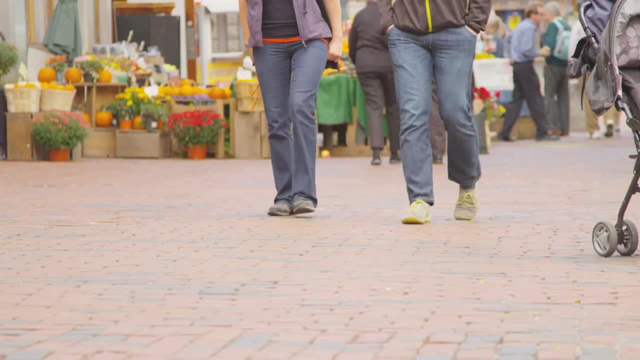 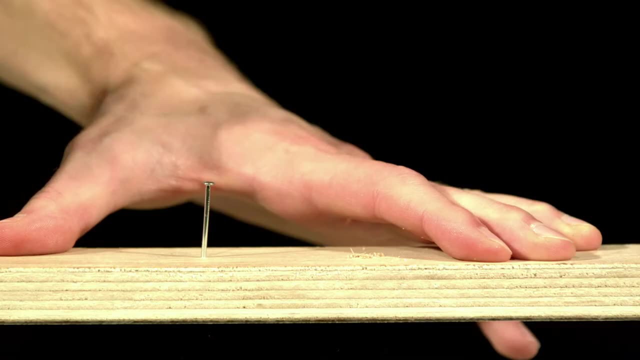 When you walk down the sidewalk, you push on the ground. the ground pushes on you. A swimmer pushes on the water. the water pushes back on the swimmer. A hammer pushes on a nail: the nail pushes back on the hammer. 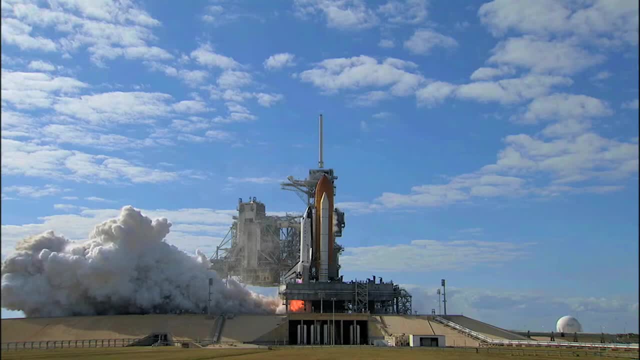 At a rocket launch, the rocket's weight- yes, weight is force- is pushing on the ground and the ground is pushing back on the rocket. an action-reaction pair. And on liftoff, inside the rocket engine, all the combustion gases are igniting. 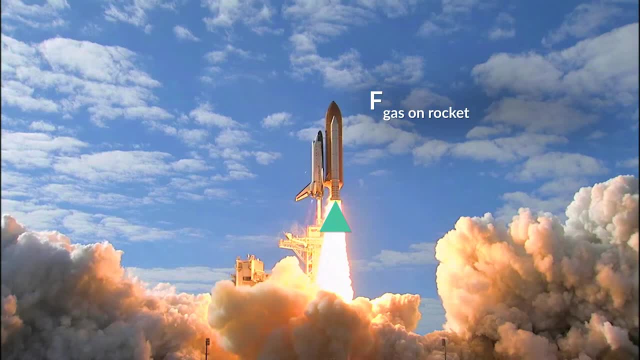 pushing on the rocket And the rocket is pushing back on the gases with a force equal in size, but in the opposite direction. Another action-reaction pair. It is this rocket-combustion-gas action-reaction pair that will cause liftoff. 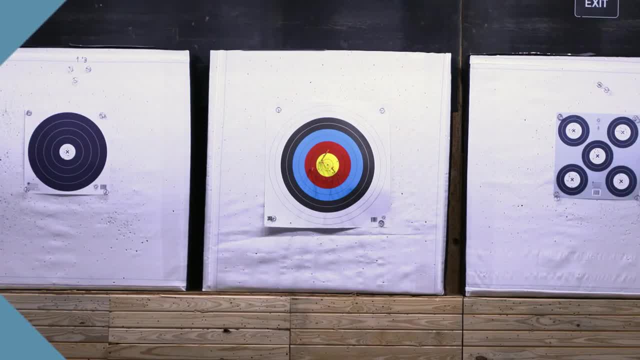 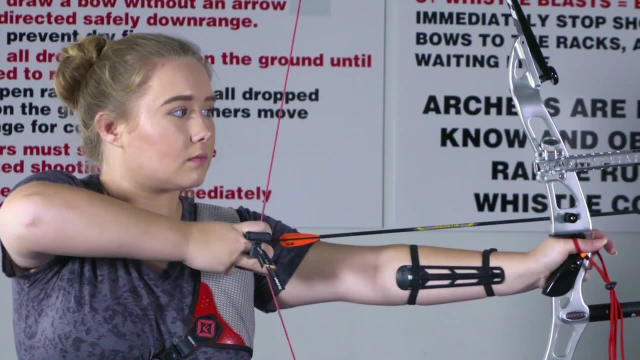 as well as the movement of the rocket into space. So let's go back to the bow and arrow. What are the action-reaction pairs that work here? There's the force of your fingers pulling back the string and the string and bow reacting.